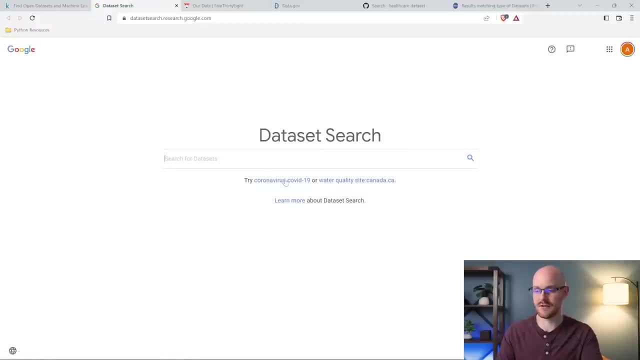 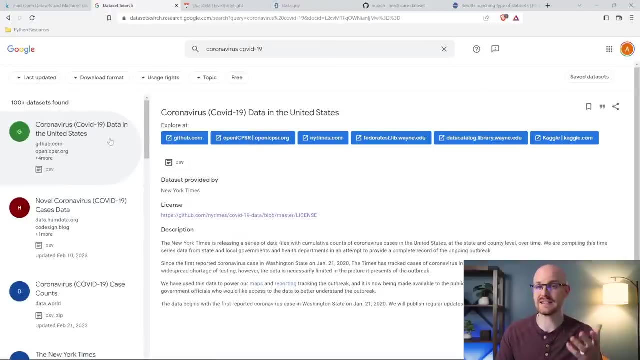 You can still search for datasets, and let's just try the coronavirus COVID-19.. It prompted us to do it, so why not? What this is going to do is it's going to search the web and find datasets for you, So then you can come over here and you can see. it's a CSV, it's a zip file. 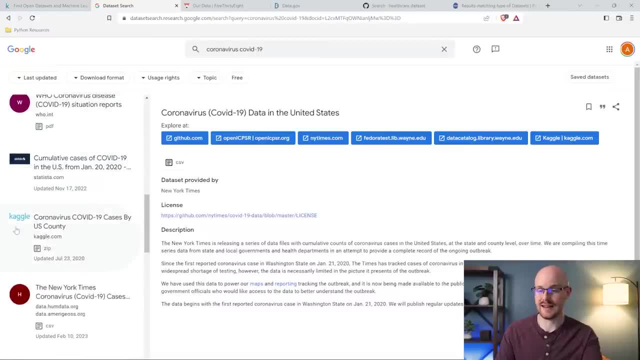 We have a PDF and they even can source in Kaggle datasets as well. But then you can come in here and you can say it found datasets and it's going to explore them. So you can find these datasets at these locations. So it's often not as straightforward. You have to do a little. 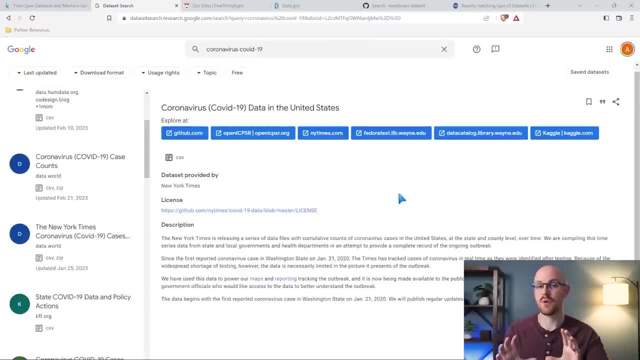 bit more digging than Kaggle, but, But typically you're getting more reliable sources of data. So with this, if you're looking for an actual COVID-19 dataset, things like data world is another kind of reputable place to find datasets, Although I think you may have to pay for some of them on some of these websites. but 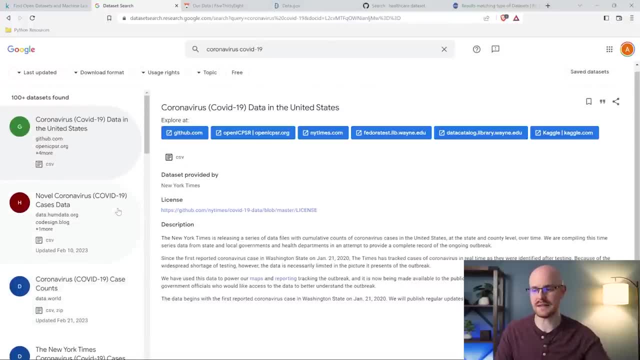 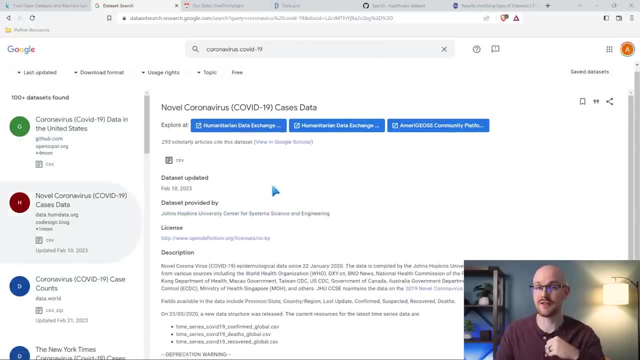 you can find datasets from the entire internet, not just one website, And that's what this is really really good for. So you may have to search around to kind of find it and then click on these links and then download it from those websites, But this is kind of an all in one place to search. 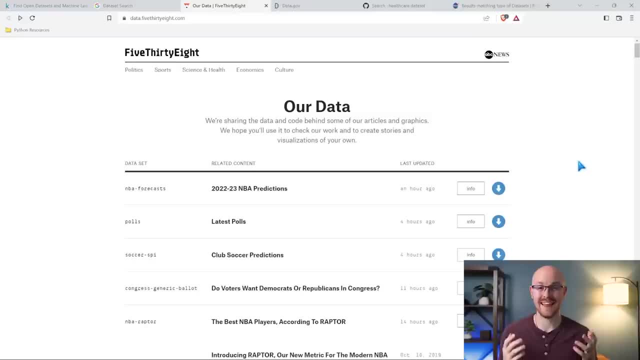 Which is really helpful. Again, just a little bit different than Kaggle. Now. the next website is called FiveThirtyEight. Now, if you've never heard of them, they're an analytical news website, So it's like a data driven website for news. I follow them every so often. I think they're 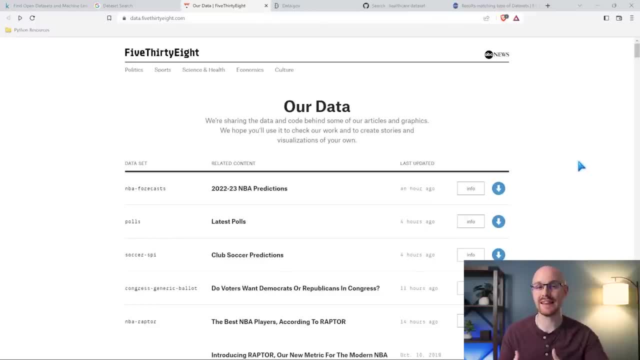 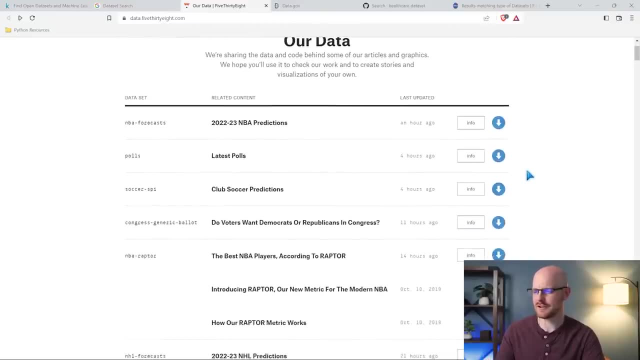 pretty cool, but they also have open access to the data that they use for their news articles, which is just really, really cool. So you can come over here and let's say, I wanted to do NHL predictions, So hockey, I'll click on this link. 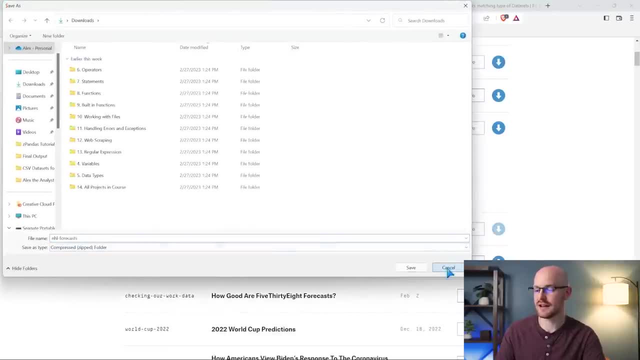 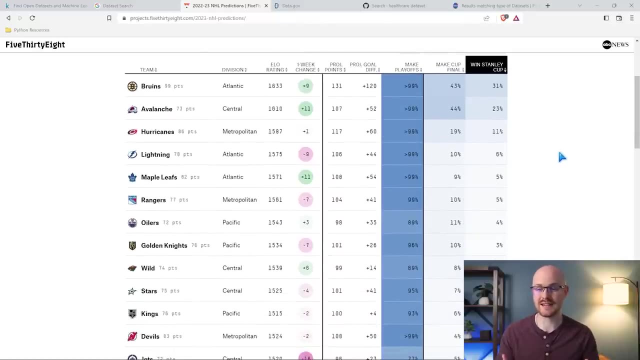 And it's going to actually download all of the data in here. Now you can click in here as well And you can actually look at the data that you're about to download, And so you can just download a lot of these free data sets, and they're pretty wide and varied, But you know. 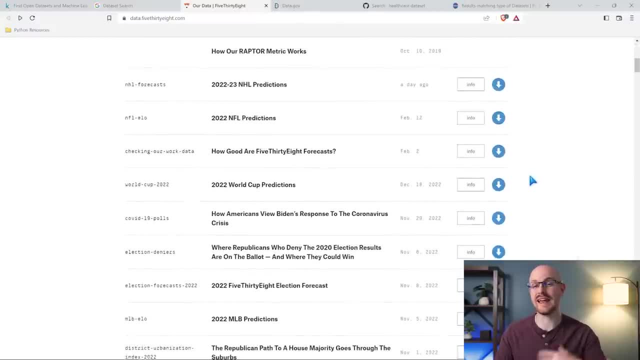 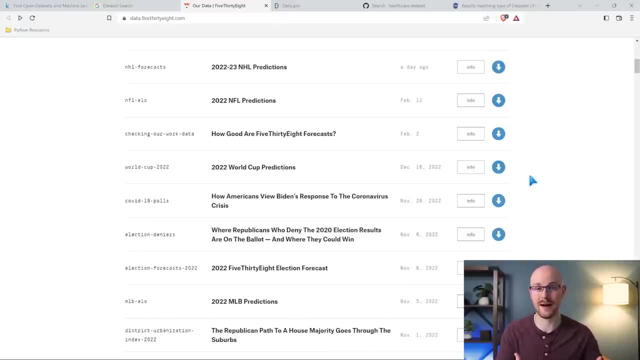 you can kind of look through and find some really, really interesting data sets. And if you find the news article, you can actually go and look at the exact data that they use and you can kind of verify what they're posting and talking about. The next website for finding data sets is datagov. Now. 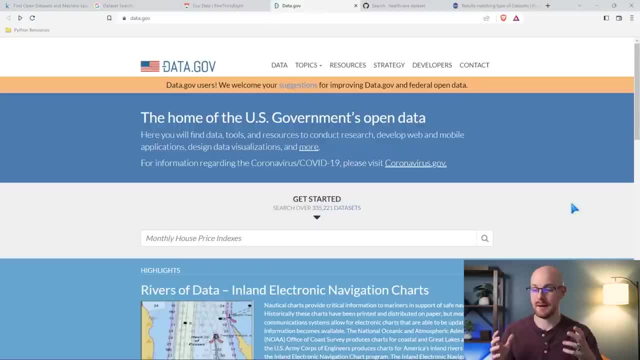 this one is for people in the US, although anybody can use it, but there should be one very similar to this for almost any local government or agency, for most countries as well. So this one is just one that I've used, but you can come in here. It can prompt you to search for things. I'll search. 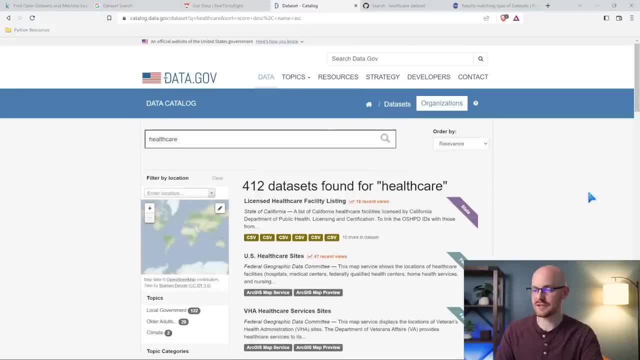 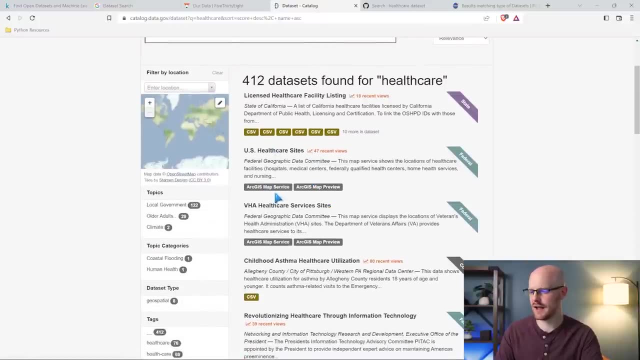 for healthcare, and what it's going to do is it's going to find all the data sets that they have on healthcare. They'll tell you if it's a CSV, if it's an API. that's not an API, But sometimes I'll have PDFs APIs. I don't know if you want to look around, but sometimes they'll give you things like: 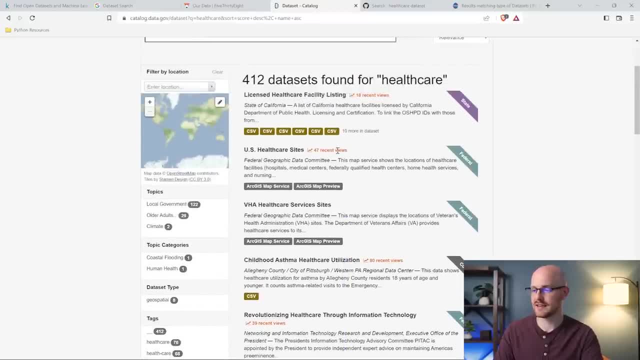 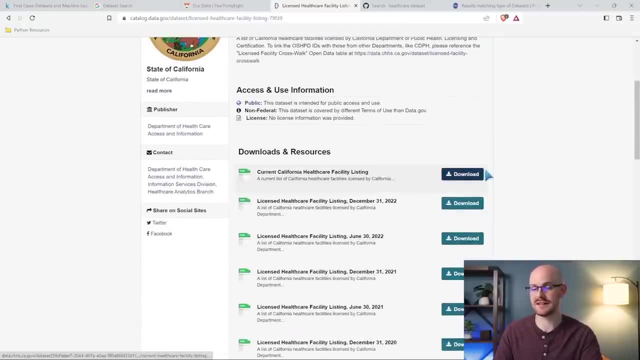 JSON XML and then you can click into these, like this licensed healthcare facility listing. this isn't a data set that I'm interested in, but then you can go and just download it. click on this and download that data set. this is definitely more government data, so for this website it's more US specific state. 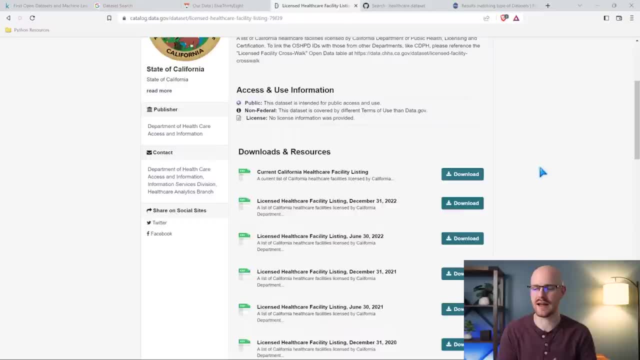 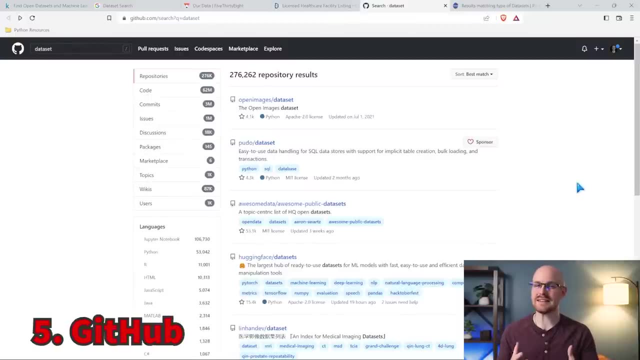 specific, local government specific or federal government specific, but they have really, really good stuff. I've used a lot of data from this website. the next place that we're gonna look is github. now, github isn't typically known for datasets, but I personally put a ton of datasets in here for free, for all my 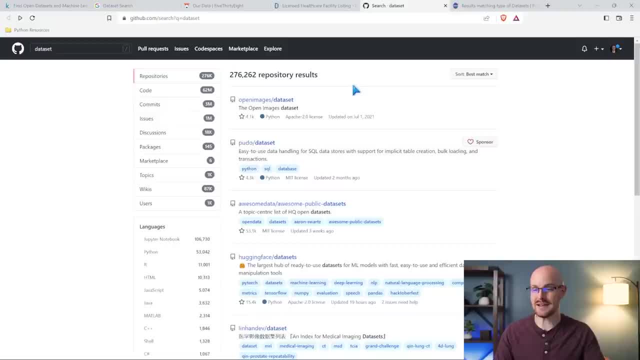 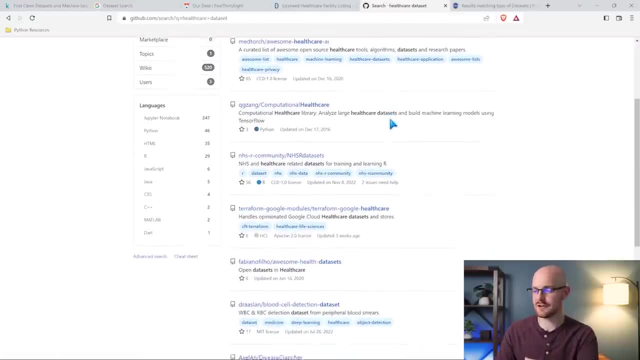 YouTube stuff, and so do a lot of other people. as you can see, if you search for a dataset in github, there's 276,000 repositories that have dataset in them. so if you want to search for something like healthcare dataset or something like that, you can scroll down and you can find stuff for that. so this one's. 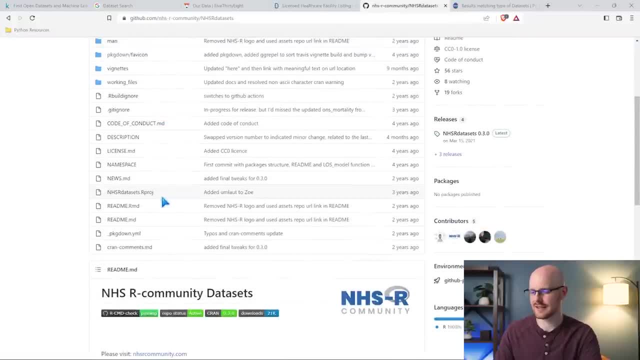 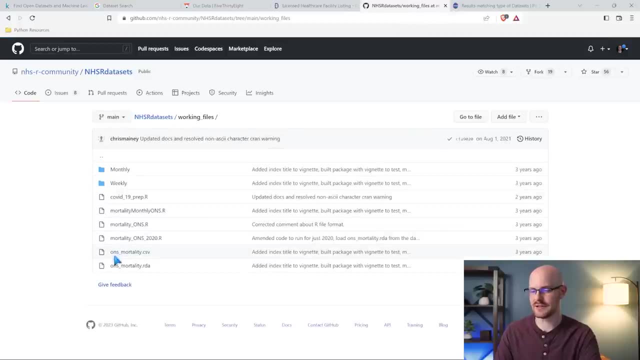 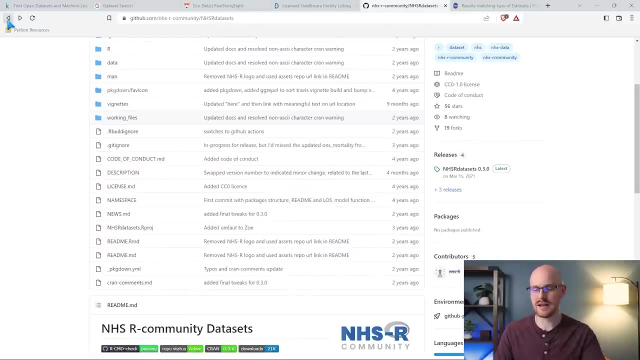 nhsr dataset sets And it looks like this one's for the R community, but we can also use that. So you just find their working files. And now here's some mortality rates with a CSV. So this one is a little bit more tricky. You have to really kind of understand how GitHub works, but I found a lot of. 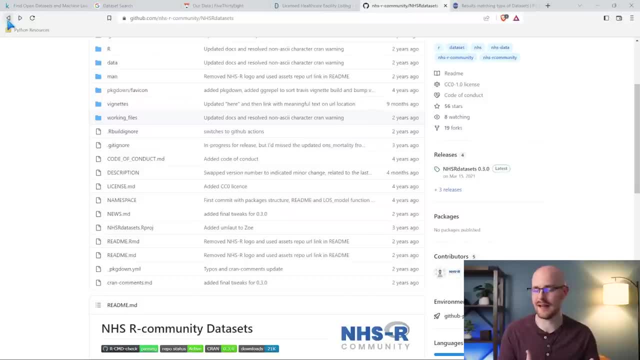 great data sets from GitHub from people who are doing projects similar to mine. So if you have a project that you want to build, you may be able to find the entire project with code and everything on GitHub, but also be able to download that data set as well. Now the last one I'm going to show.